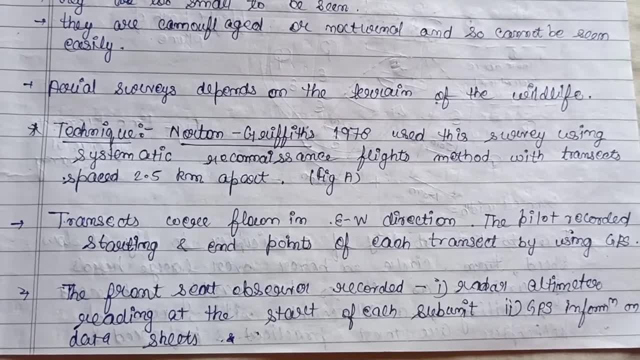 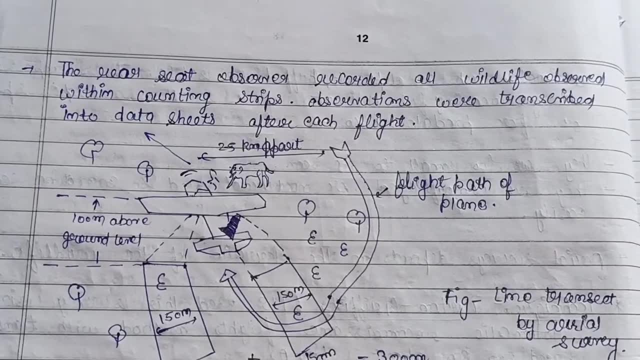 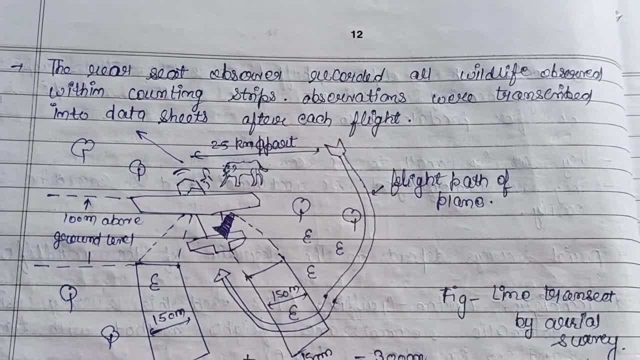 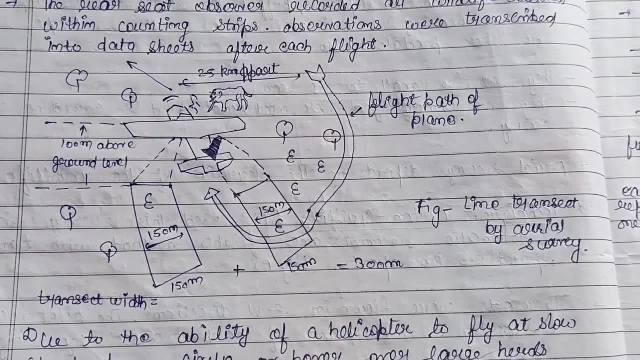 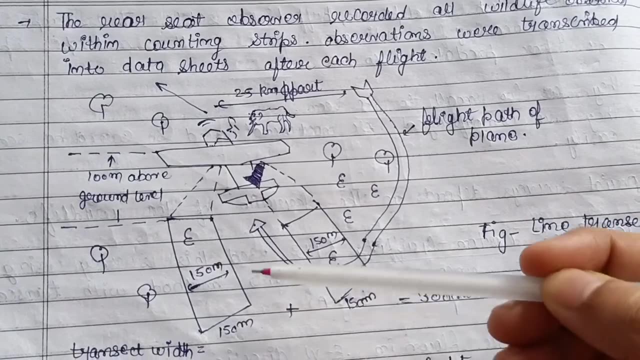 Observations were transcribed into data sheets after the each phase, So basically after the observation data is recorded. So this is a diagram that is line transact by the aerial survey. So here, so here, this is the actually the path route of the flight if an animal is observed. 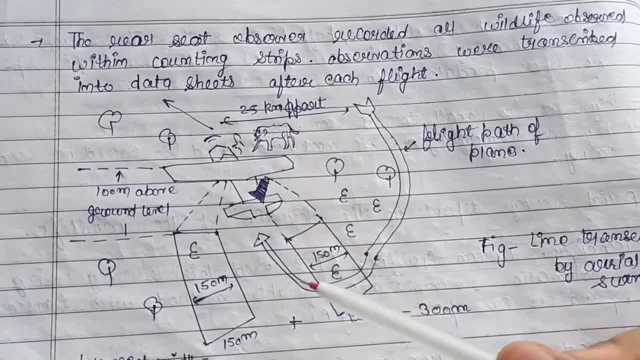 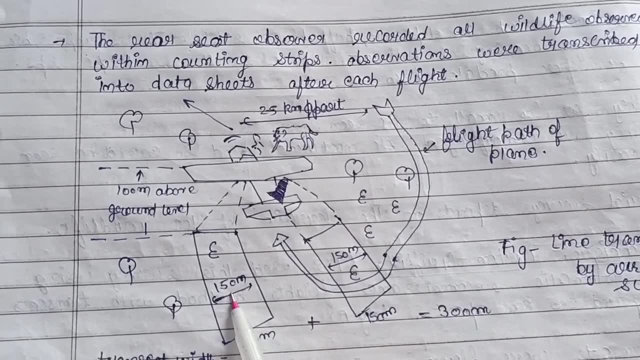 here. so it is marked by that. these are the transacts that are laid down, that is, in east direction and west directions. okay, and this is the we can say the width between the transact, that is 150 meter. 150 meter, that is the total of 300 meter. 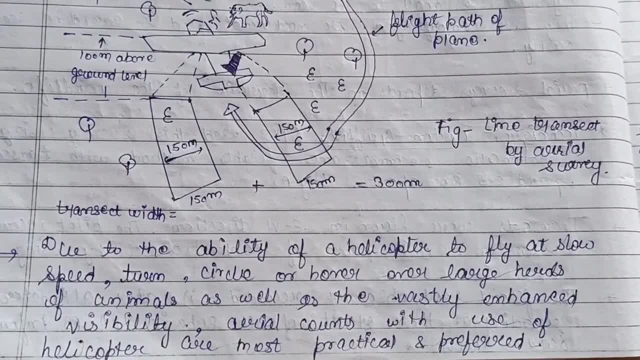 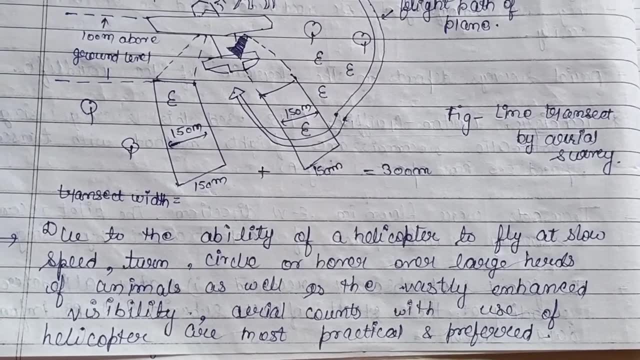 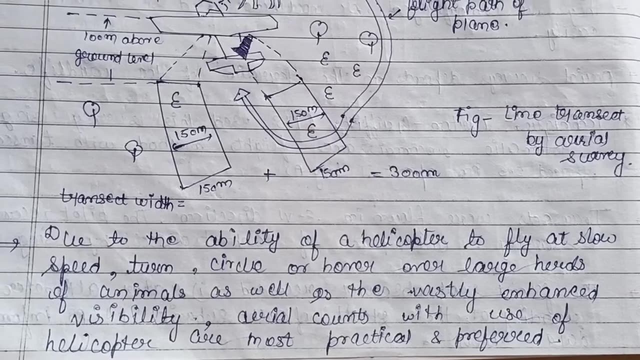 So, due to the ability of a helicopter to fly at the slow speed, Turn, circle or hover over the large herds of animal, as well as the vastly enhanced visibility, aerial count with the use of helicopter are most practical and preferred. so, basically, helicopter is used in this method. 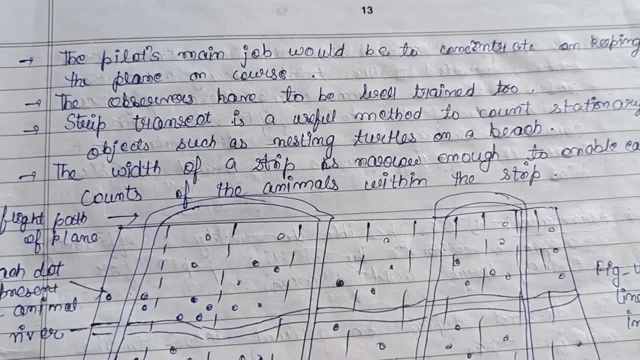 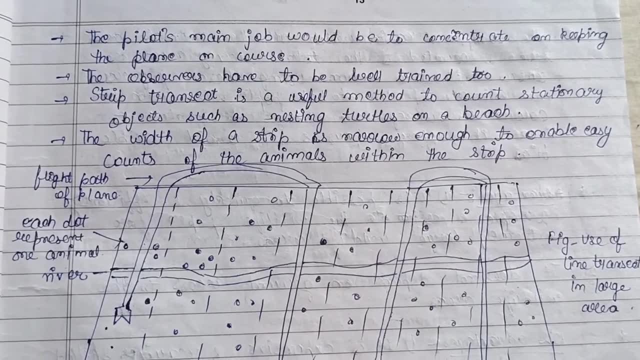 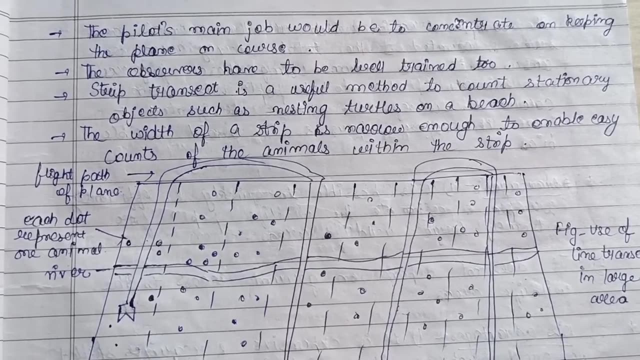 The pilots main job would be to concentrate on keeping the plane on course that is, in right direction. The observers have to be well trained too, so that they will notice the particular animal, a step transact. It is a useful method To count The stationary objects, says the nesting turtles on a beach or plants. we can say 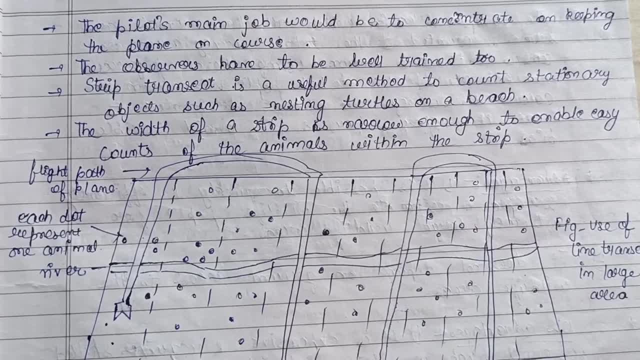 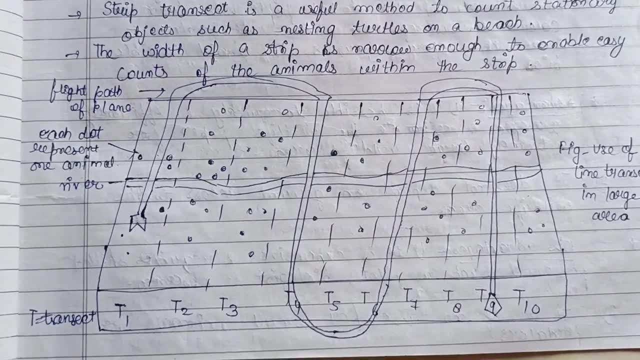 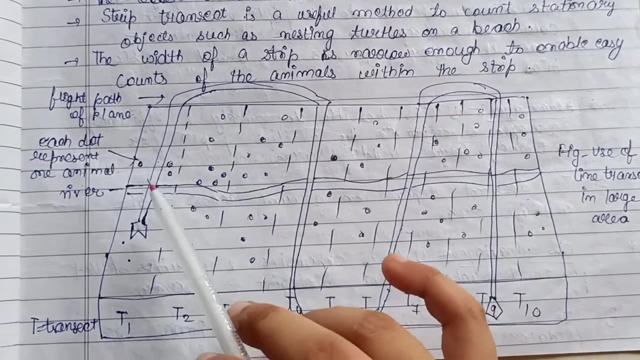 So the width of a strip is narrow enough to enable the easy count of the animal within the particular strip. So this is a diagram that is use of line transact in a large area. here t denotes transact, that is t1, t2, t3, t4, t5 respectively. we have drawn here and flight path of the plane. that should.